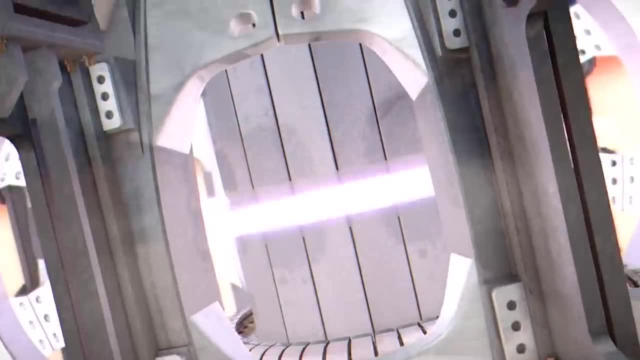 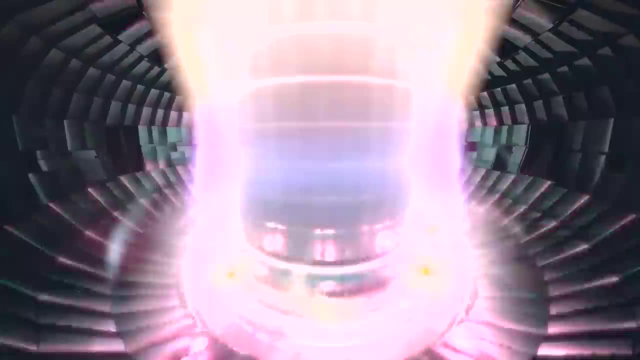 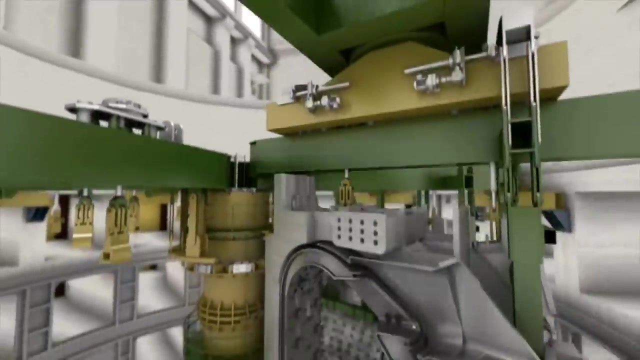 in a tokamak reactor. These hold the extremely hot plasma in a shape which famously resembles a donut, known as a torus. The plasma is confined into this shape using powerful superconducting magnets which prevent it from burning the walls of the reactor. Inside the plasma, the best fuel 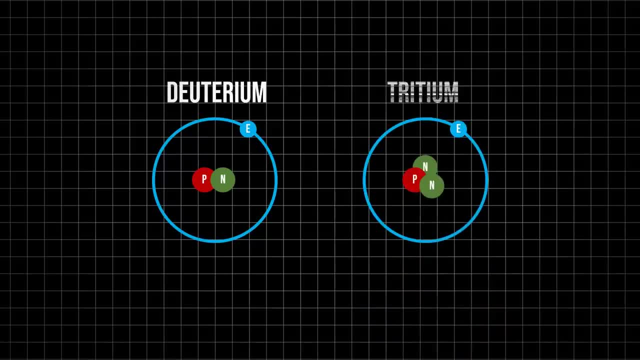 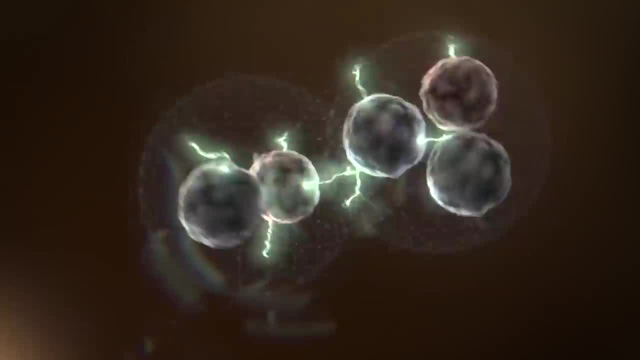 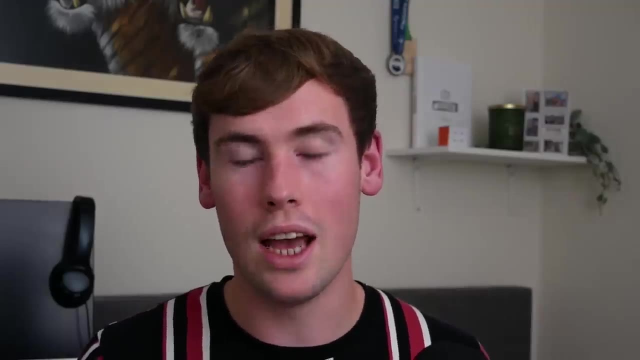 mix is generally a blend of deuterium and tritium, which are special forms of hydrogen known as isotopes. Given the correct conditions, these atoms will overcome their repulsive forces and fuse together, releasing energy, in the process, However reaching reliable and economic nuclear 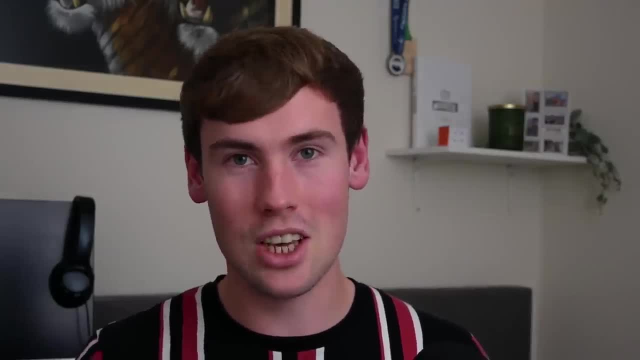 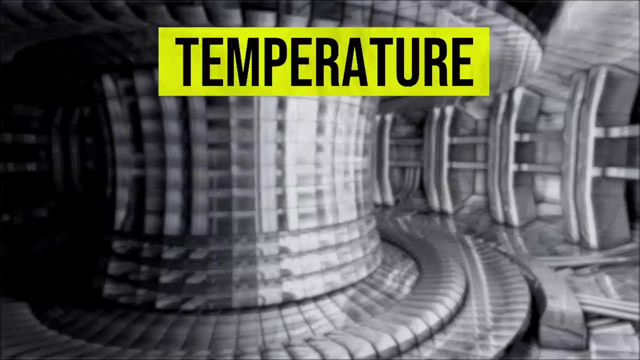 fusion has a fair few challenges, giving scientists an array of possible problems to solve. Arguably, the main four challenges for nuclear fusion are: reaching high plasma temperatures. enabling high fuel densities within the plasma. suitably confining the plasma within the reactors. 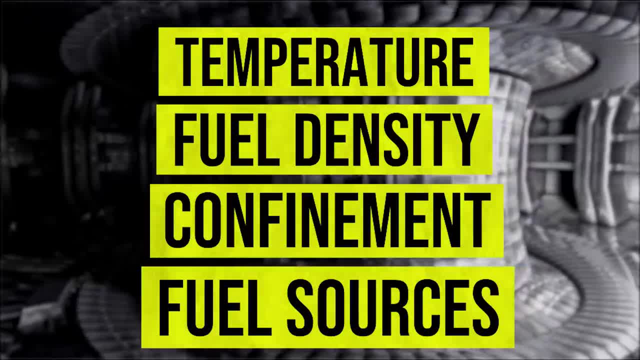 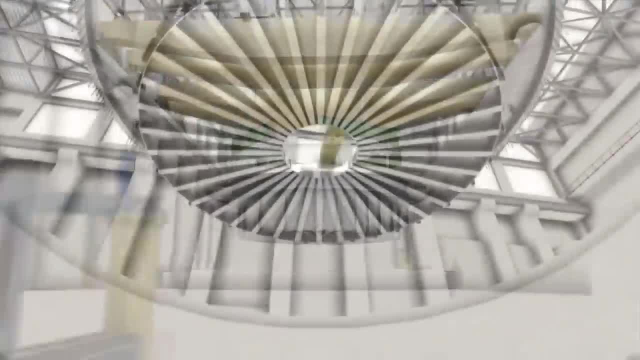 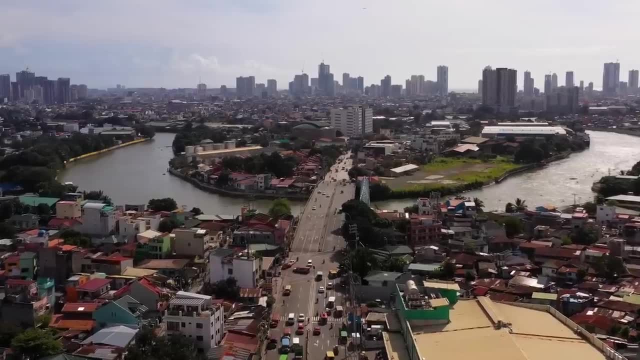 and ensuring there is a sustainable generation process of fuel for the reactors to use. When all of these considerations are achieved successfully, nuclear fusion can take place in such a way that it could become commercially viable to capture energy and power civilizations around the planet. The first three of these challenges are summarised in something called the triple product, which 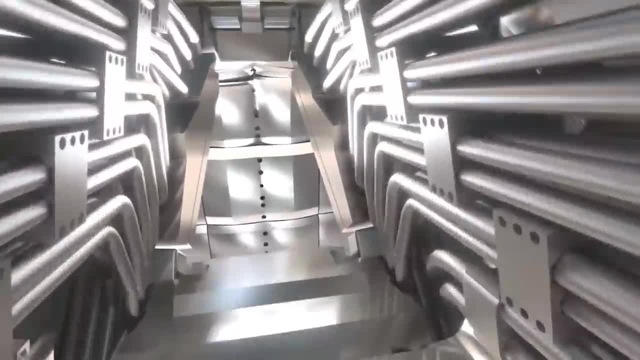 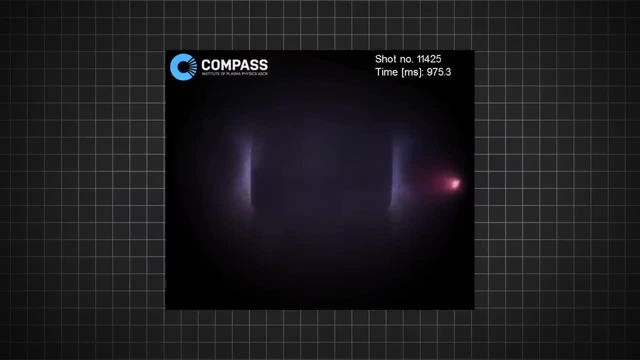 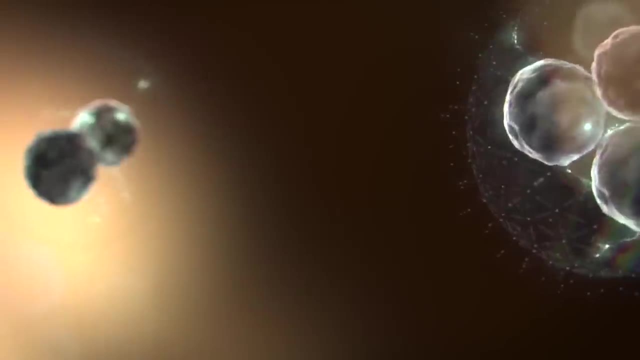 is a value that scientists want to maximise because it indicates how feasible a nuclear fusion reactor is. A high enough triple product will mean a tokamak reactor can release enough energy to make it operational as a power plant. Generally, this is seen as the point at which 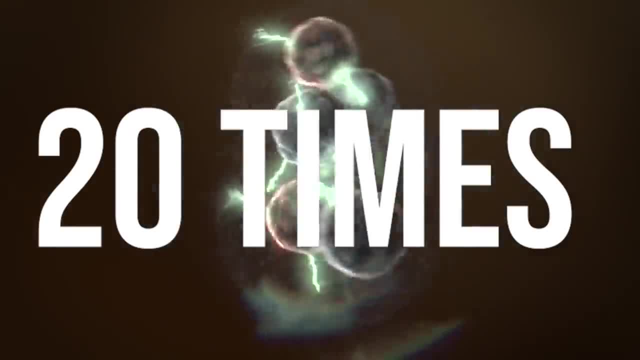 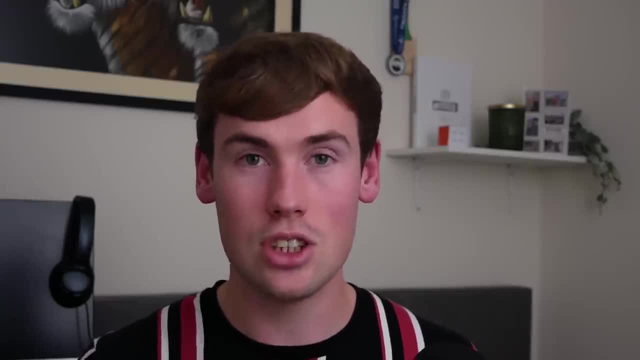 the fusion reactions release 20 times as much energy as was used to heat the plasma up up. For tokamak reactors, about 150 million degrees celsius is generally seen as the best operating temperature. This is because it requires the lowest combination of fuel density. 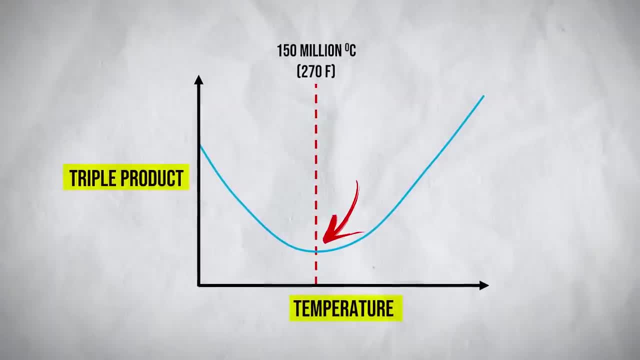 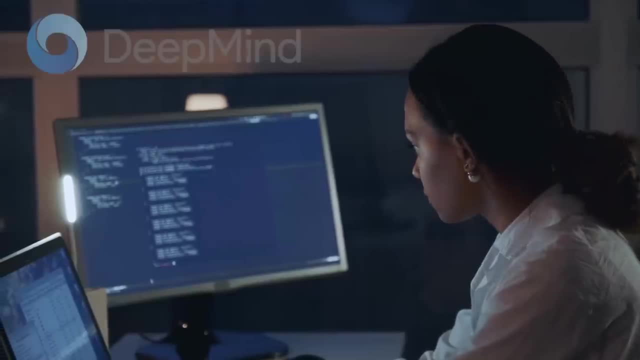 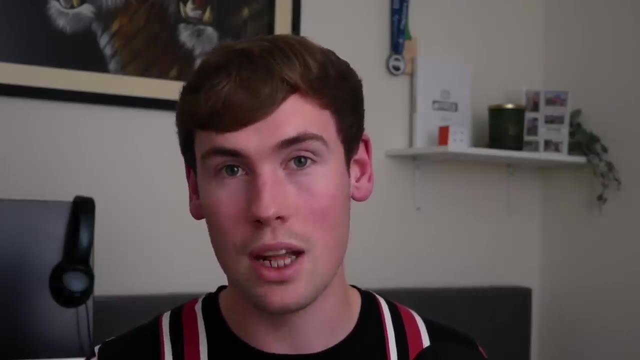 confinement, quality and temperature to operate as a commercial reactor. However, getting all of these values high enough is yet to be done. Therefore, Google's deep mind is trying to offer their skills into the mix. Specifically, they are trying to help the quality of plasma confinement. 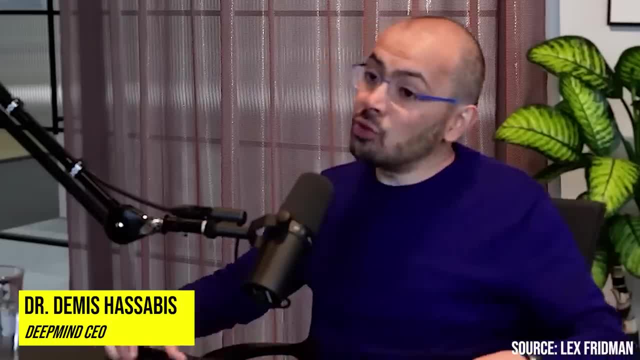 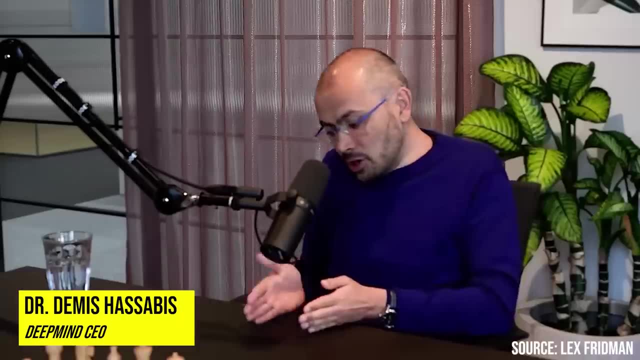 What we tend to look at is, if we go into a new domain like fusion, what are all the bottleneck problems like thinking from first principles, you know what are all the bottleneck problems that are still stopping fusion working today. And then we look at those bottlenecks and 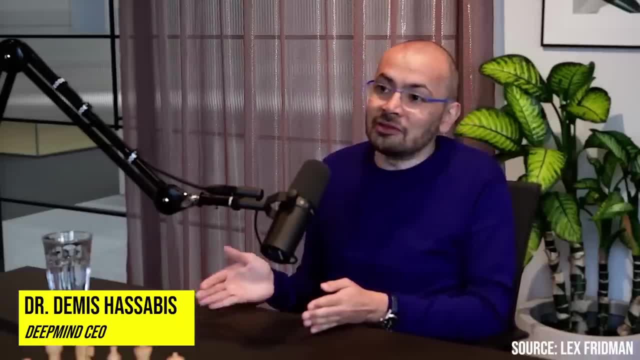 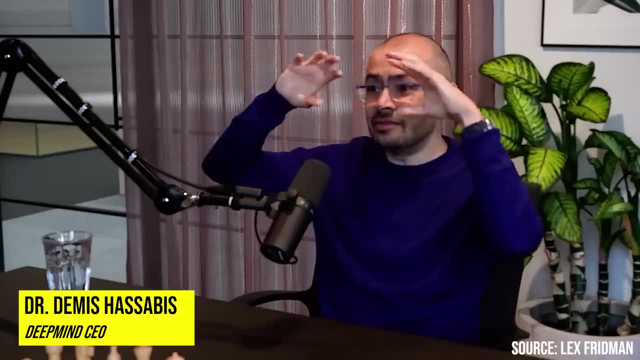 we look at the ones, which ones are amenable to our AI methods today, And in this case, plasma control was was perfect. So you know, the plasma is hotter than the sun and there's obviously no material that can contain it, So they have to be containing these magnetic 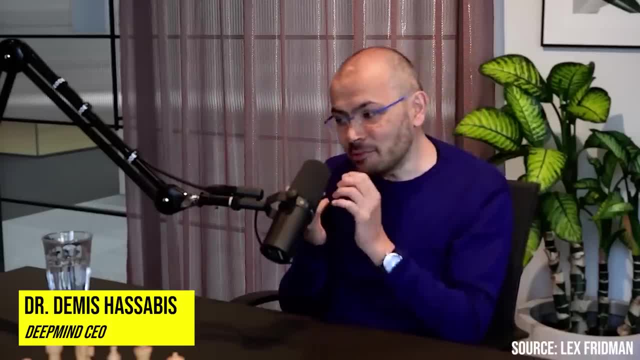 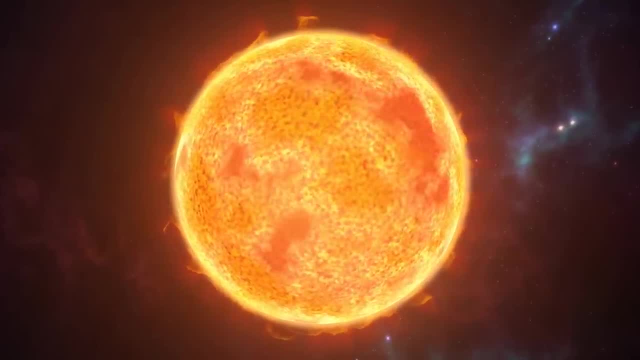 very powerful metal Plasma, superconducting magnetic fields. But the problem is plasma is pretty unstable. As you imagine, you're kind of holding a mini sun, mini star in a reactor. So you know you kind of want to predict ahead of time what the plasma is going to do. so you can 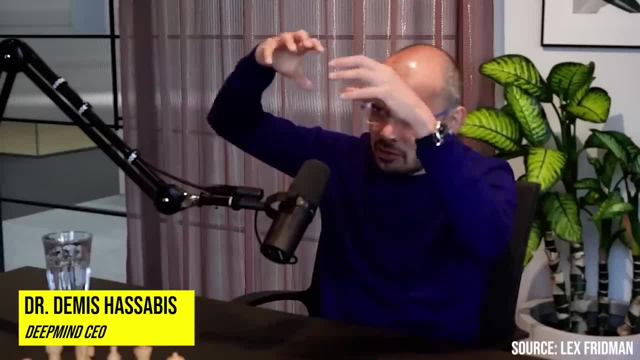 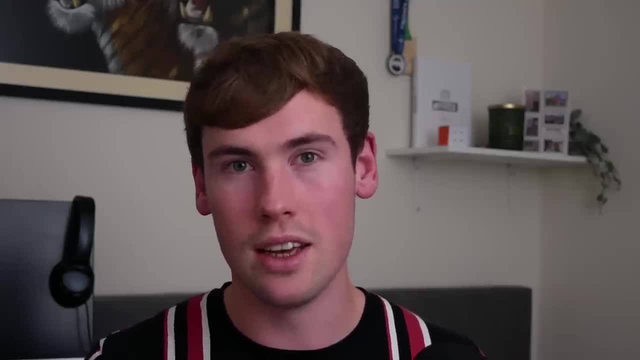 move the magnetic field within a few milliseconds, you know to, to basically contain what it's going to do next. The method used by DeepMind that led to this breakthrough is called reinforcement learning. This is a type of machine learning algorithm that learns by being rewarded for. 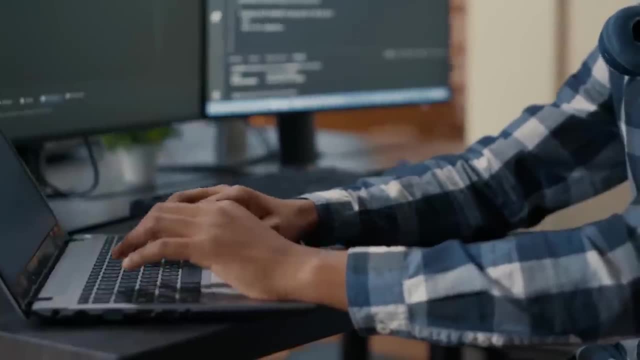 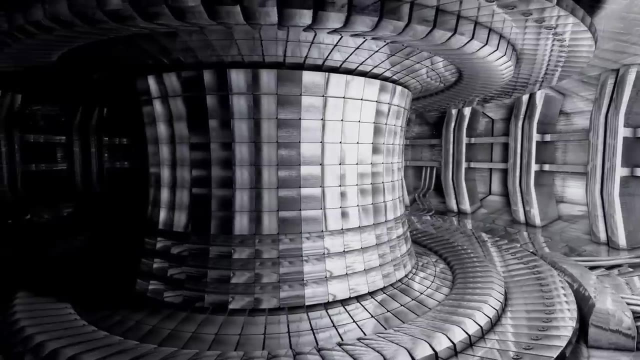 making decisions that we want and punished for making decisions we don't want. This is similar to how you might train a dog, But instead of a dog it's a fusion reactor, And instead of a brain there's a deep neural network. 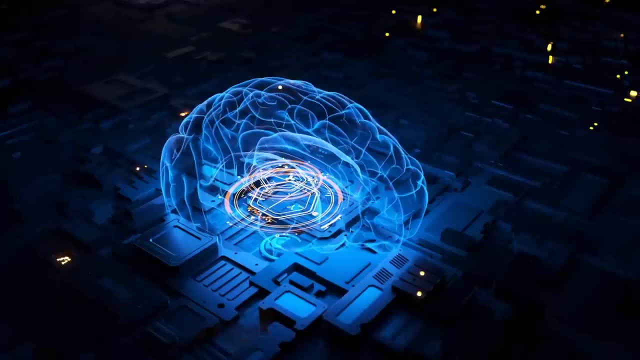 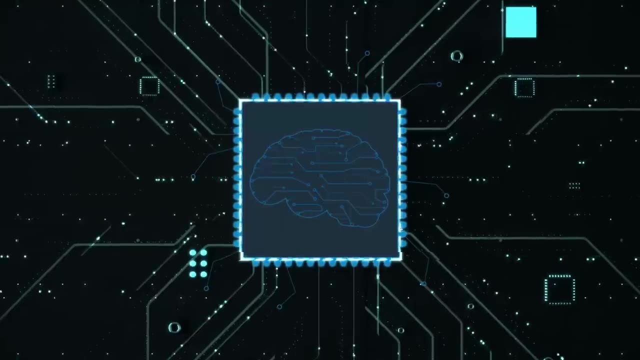 In a fusion reactor, for example. this would mean we reward the machine learning system when it makes the superconducting magnets hold the plasma in the desired shape. Likewise, rushed fusion. if the machine learning system makes a mistake and the plasma becomes useless, this can do. 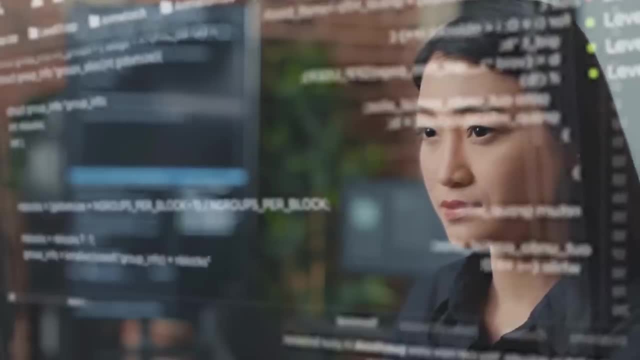 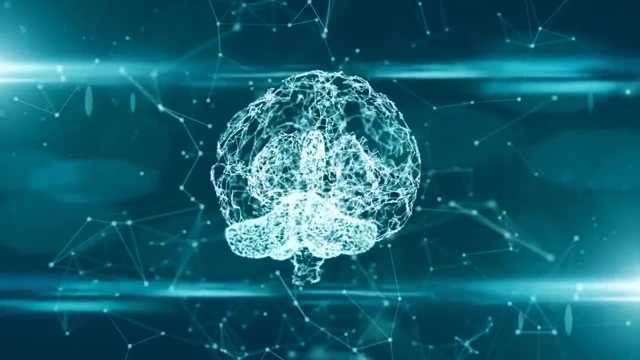 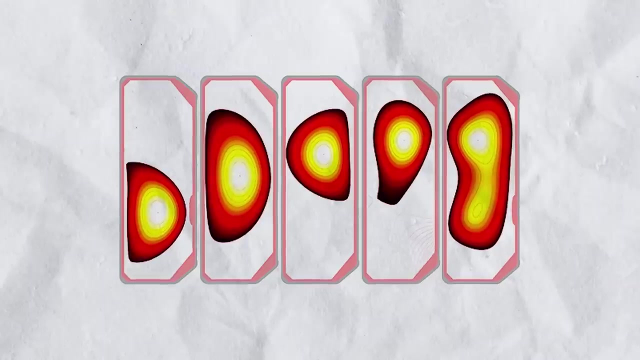 becomes unstable and breaks down, it will be mathematically punished. So what does this look like in practice? The reinforcement learning model was set to learn how to hold plasma in a number of different shapes. This is important, as some shapes that are very difficult to make are actually better. 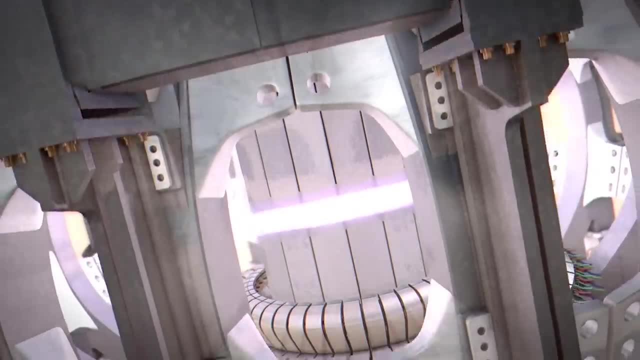 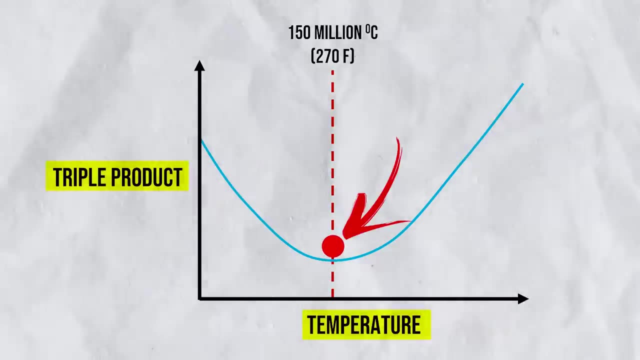 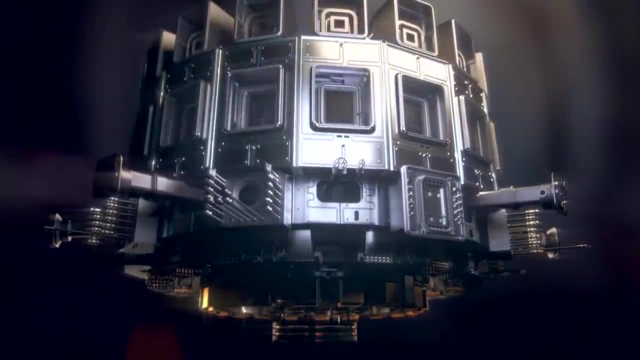 at containing the energy within the plasma. This means that if we can create these shapes, we can improve the confinement quality of the plasma and therefore increase the triple product, bringing the dream of nuclear fusion slightly closer to reality. This confinement quality is measured by the energy confinement time and represents how 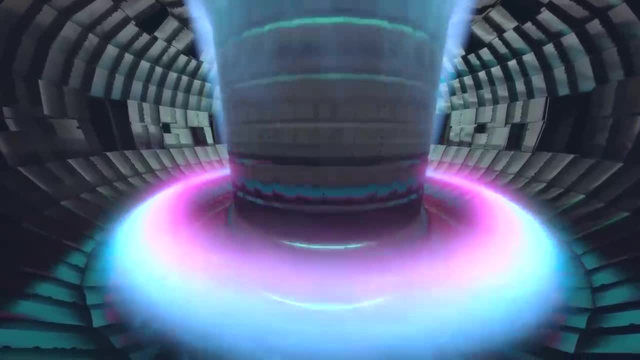 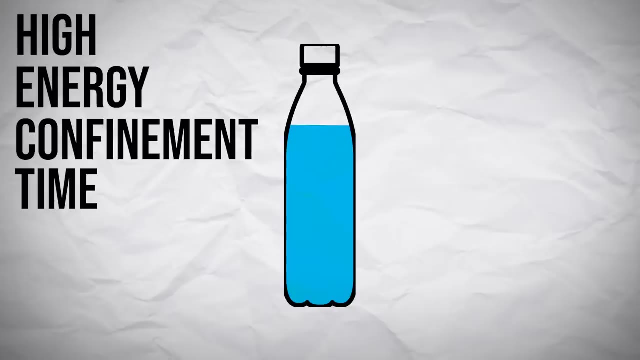 quickly the plasma loses energy to its environment. The analogy of this is that if the nuclear reactor was a bottle of water, it would have a high energy confinement time if it was good at keeping the water in, But if it had lots of holes in it and was leaky it would have 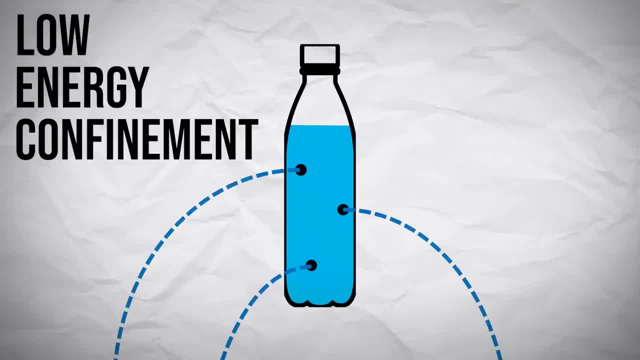 poor energy confinement, but it would still be able to keep the water in. So yes, thearlai Jesus does not reveal a high她ателяe plate in this video is officially been put in launch pad, but it does not reveal how many channels it can apply to. 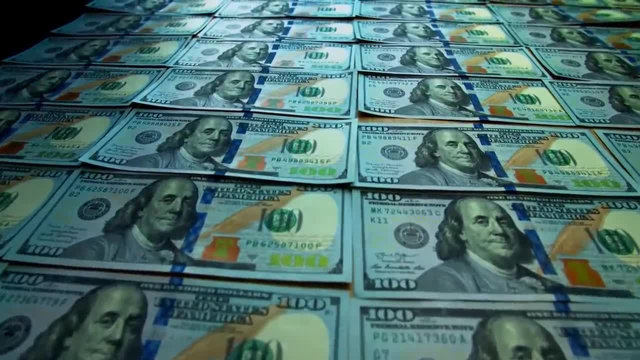 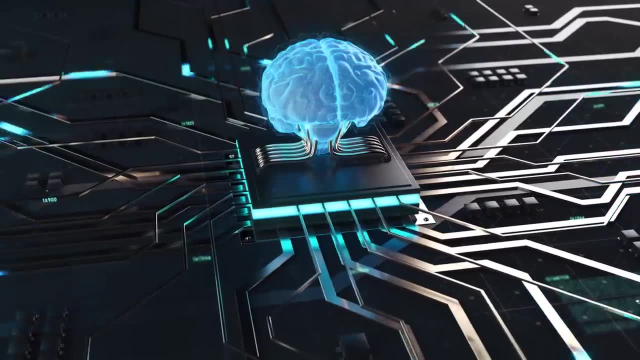 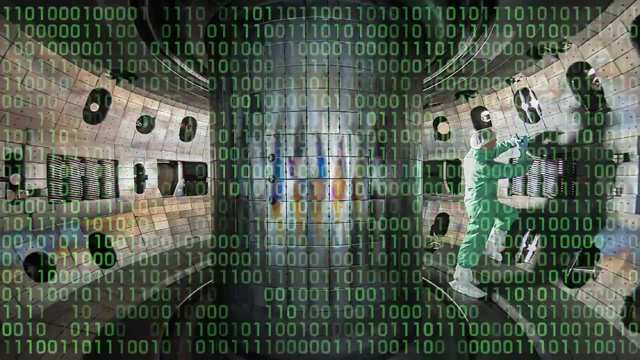 Unfortunately, operating a nuclear fusion reactor is currently extremely expensive. Therefore, it isn't possible to run it for long enough for the artificial intelligence to learn how to confine the plasma in the required shapes. Therefore, the model was actually trained on the simulation of the reactor before being put to action on the 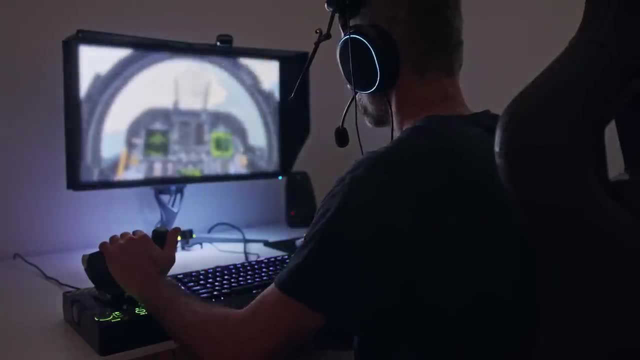 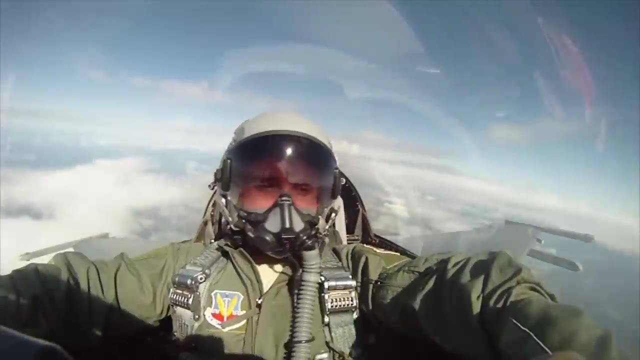 real thing. This is similar to a pilot training on a flight simulator before flying a real plane, as it is much cheaper to do and mistakes are much less expensive. After a number of days of training, it was time to see how it actually performed on the. 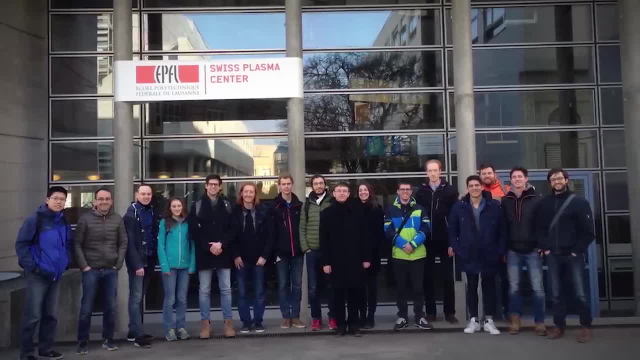 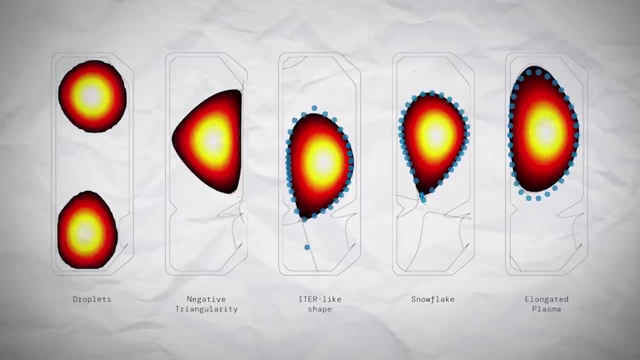 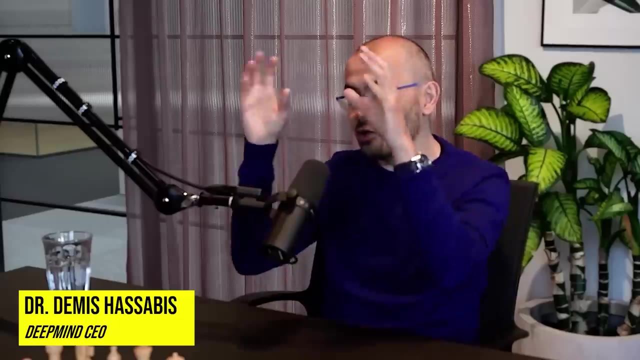 real reactor owned by the Swiss Plasma Center. If we take a cross section of the fusion reactor, we can see the strange shapes that DeepMind managed to recreate. We held the plasma in specific shapes, so actually it's almost like carving the plasma into different shapes and hold it there for a record amount of time. 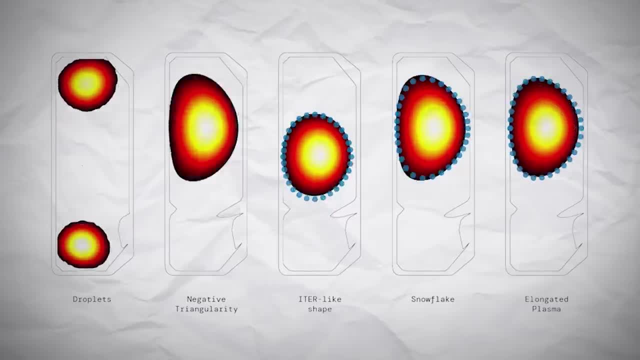 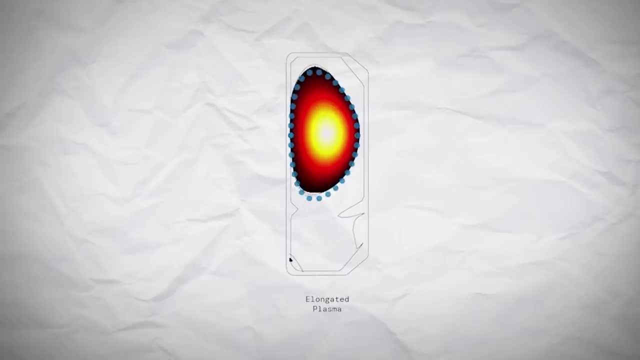 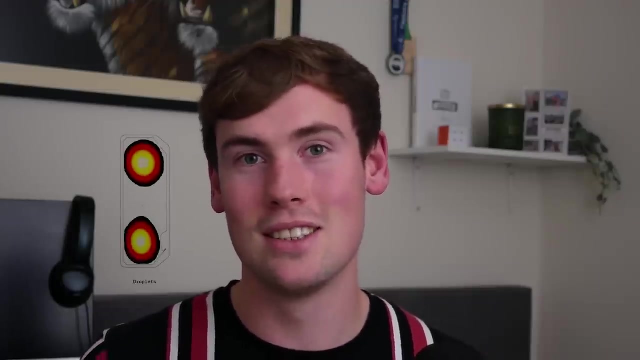 Although the exact performance benefits of these different shapes is still an open research question, the elongated plasma on the right is generally thought to be beneficial at increasing the energy confinement time of the plasma. However, my favourite is the two droplets known as doublets. 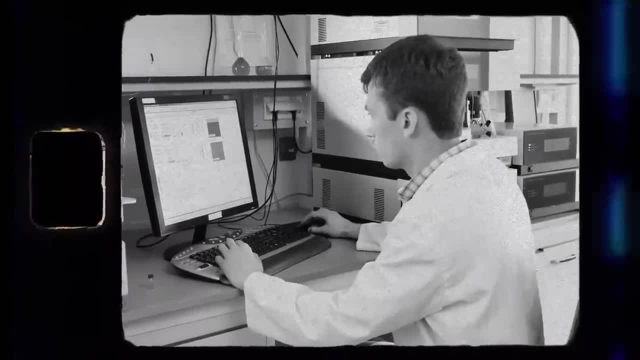 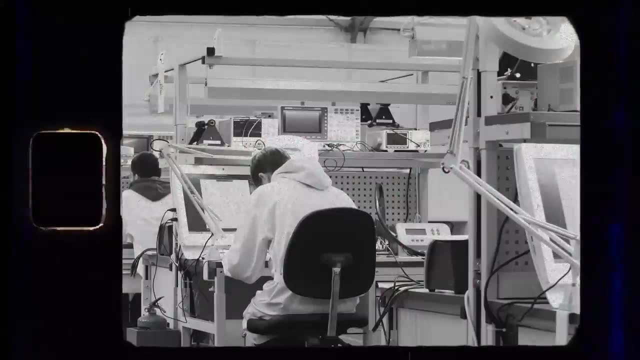 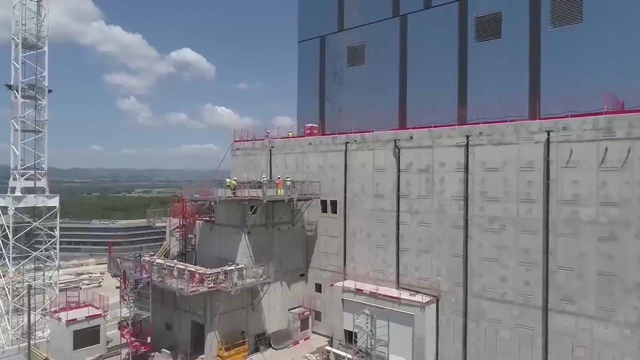 This method was actually invented in the 1970s by a group of researchers from the American energy company General Electric. After a number of iterations, this eventually led to the D-shaped plasma used by ITER, which is one of the largest fusion projects to date. 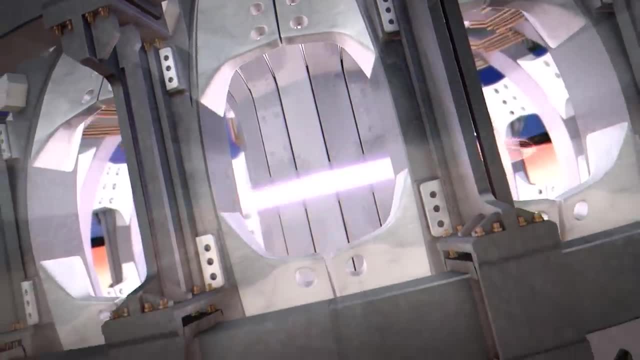 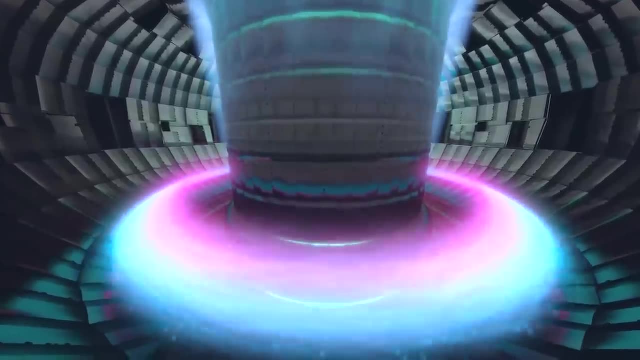 The D-shape was developed due to the difficulty holding the doublet's shape, but now, due to reinforcement learning, the doublet shape may be possible and could allow for higher quality plasma confinement. Recreating these shapes is a huge breakthrough for nuclear fusion, as it brings us ever so.